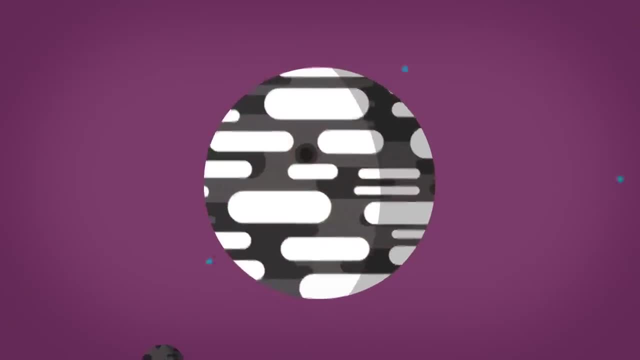 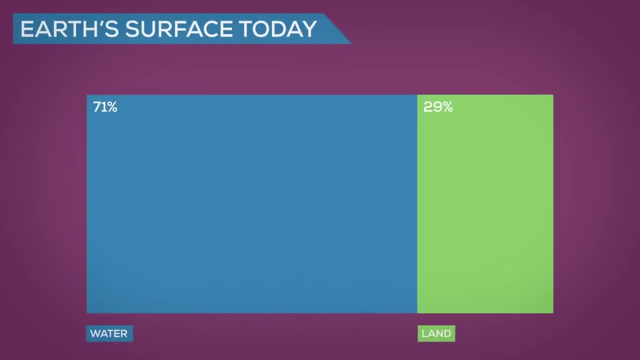 Millions of asteroids brought more and more water to our planet. All the water on Earth has about this volume. compared to Earth Today, the surface of Earth is water and 29% land. 97.5% is saline water, while only 2.5% is freshwater. The freshwater is 69%. 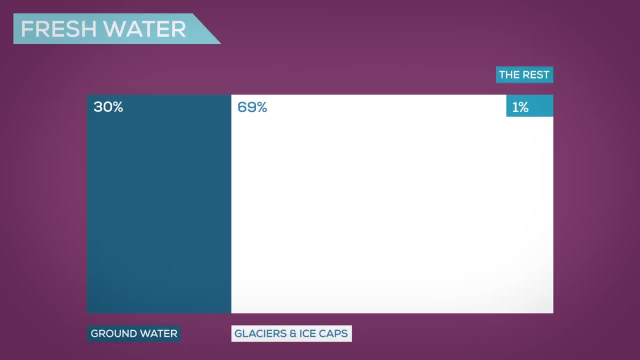 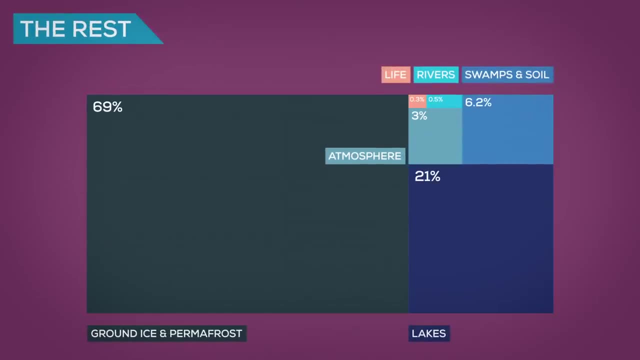 ice and snow. 30% are groundwaters and only about 1% make up the remaining groundwaters. But even this small part is mostly frozen. Only a tiny part of our water is actually lakes and rivers, and an even tinier part is bound in living things. So gradually the earth cooled down. 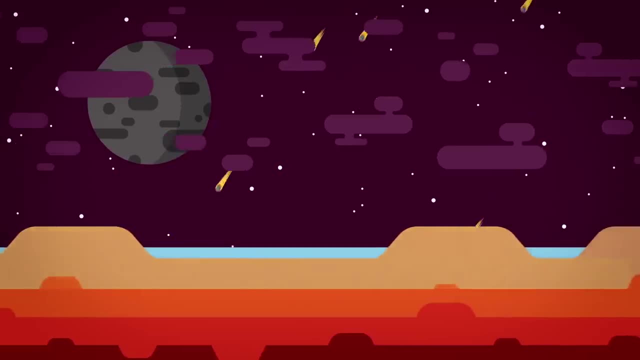 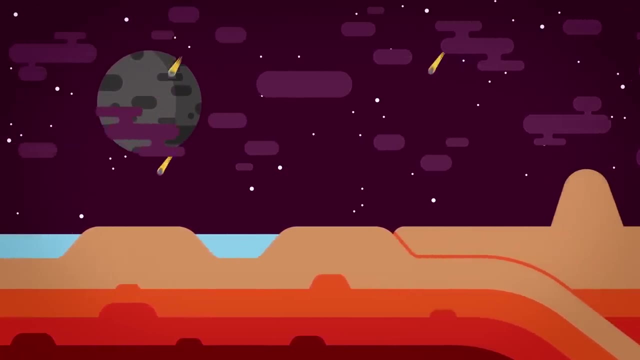 and the surface formed a thin crust, But inside the earth, hot rock continued to swirl about, moving the crust from below and breaking it apart. This process is called plate tectonics and is happening right now. We'll make a whole video about it in the future. 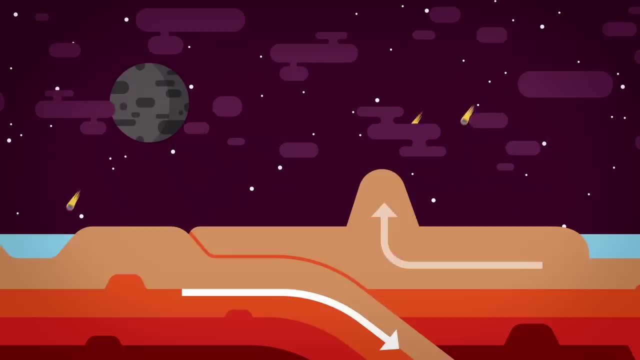 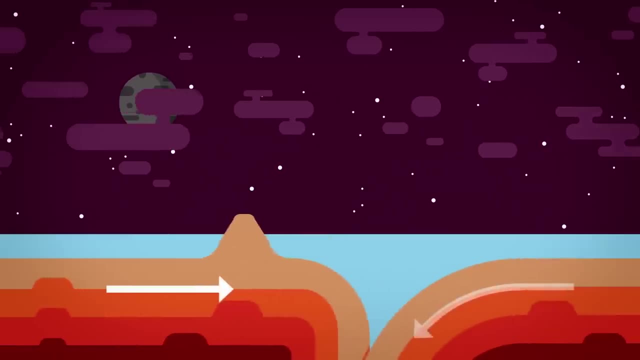 For now, let's just say that the crust of earth consists of separate giant plates that move around. As they meet, they crumble and create mighty mountains, Or violently plunge back down deeper into earth, creating deep trenches. That's the way the highest place on earth was formed- Mount Everest- and the deepest. 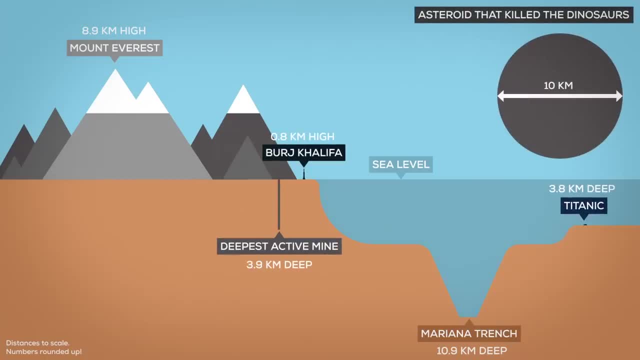 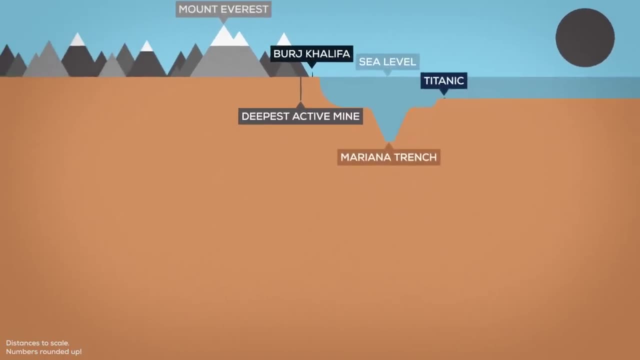 the Mariana Trench. From our perspective, earth's mountains and trenches are mighty indeed, but when you look at the earth in cross-section, you can see how tiny they actually are. The part we stand on is the crust, which is about 50 kilometers thick, though it can vary between 5. 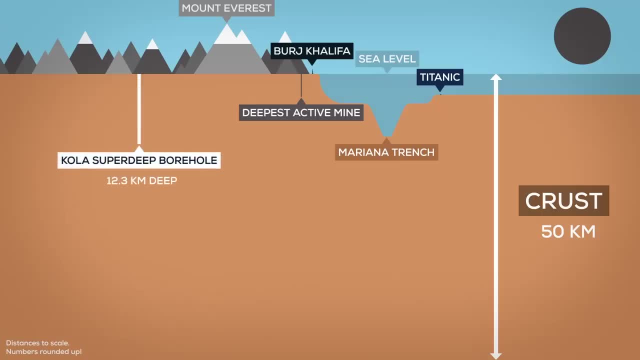 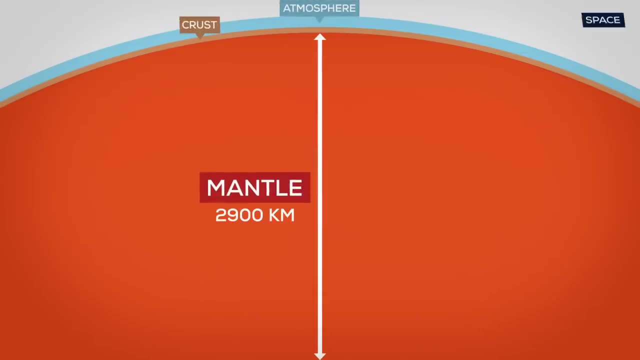 and 70 kilometers. By the way, the deepest hole ever drilled by man is 12.262 kilometers deep. After the crust comes the mantle. The mantle is a rocky shell and about 2,900 kilometers thick. The mantle consists of the upper mantle and the lower mantle. 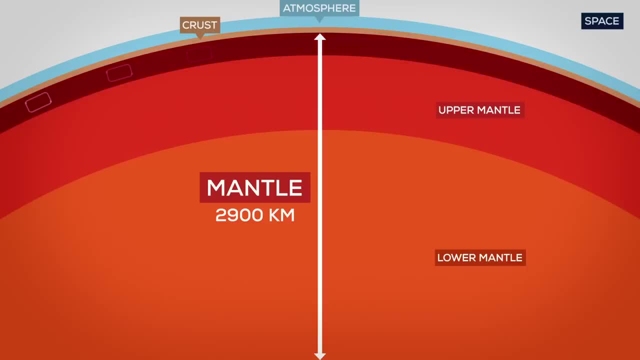 The upper mantle has different regions too. Its upper part, which is viscous and carries the crust, is called the lithosphere. After that there comes the asthenosphere, which consists of less mobile, mostly solid material. The lower mantle reaches deep down to the outer core of earth. Earth's outer core is a liquid layer of iron and nickel about 2,266 kilometers thick, Temperatures vary from 4,000 degrees Celsius to 5,700 degrees Celsius, And in the center is the inner core. It's mostly solid, a ball made of an iron-nickel alloy with a radius of about 1,200 kilometers. 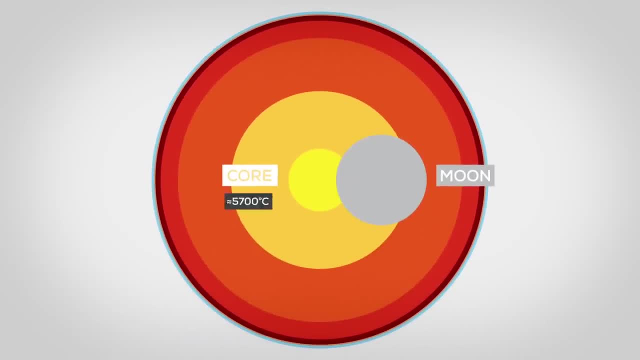 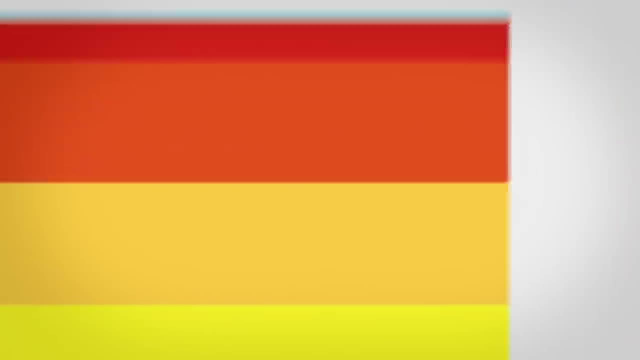 70 percent the size of the moon and about the temperature of the surface of the sun. It is slowly growing, at an estimated rate of about one millimeter per year. Now for some perspective. This small layer of crystallized milk product, which is made of iron and nickel, is made of iron and nickel. 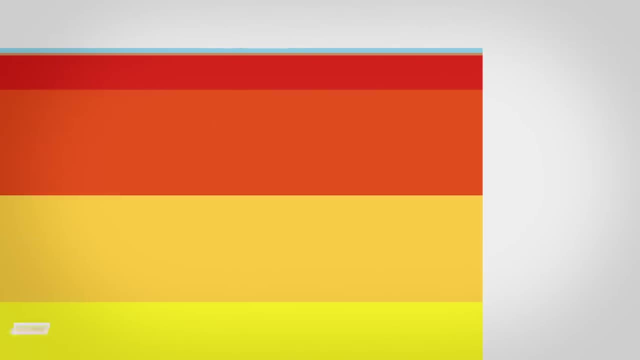 This small layer of crystallized milk product, which is made of iron and nickel, is made of iron and nickel. This small layer of crystallized milk product which is made of iron and nickel And the rocks of former molten mantle is where we live. 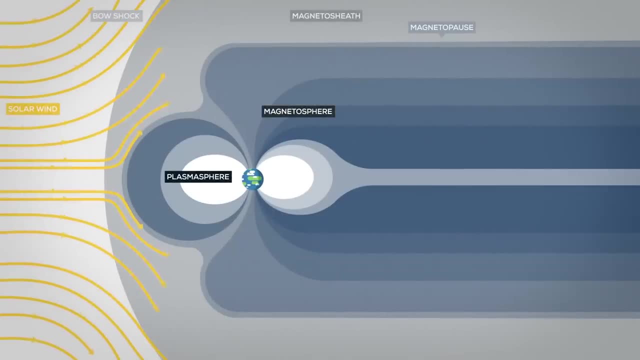 Then there's the Earth's magnetic field. It's an invisible phenomenon that diverts high energy particles coming from the sun and other sources, allowing for a stable environment with comparatively little radiation impact on earth. But why is it there? Actually, we don't really know a terrible lot about that. 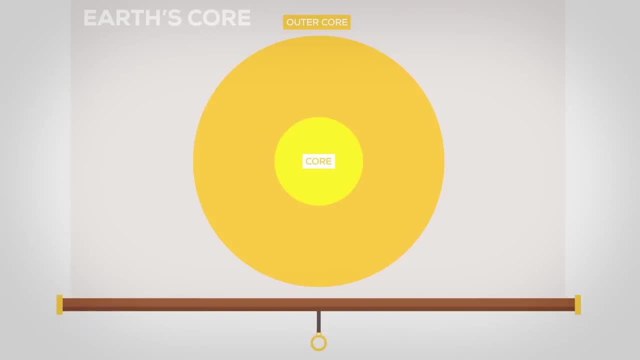 We know it has something to do with the core of the earth. Inside this metal sphere, large electrical currents flow in complicated patterns. They cause a magnetic field that sort of stabilizes itself according to the laws of electrodynamics. This entire system is called the dynamo. 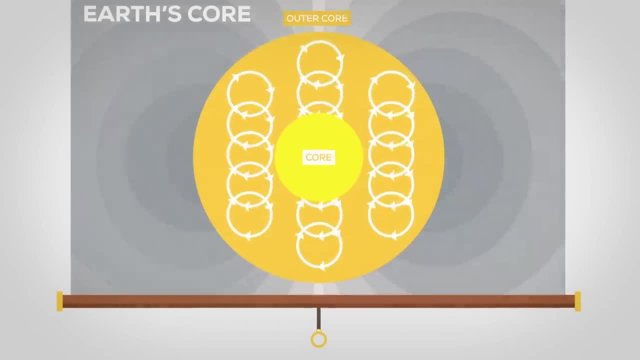 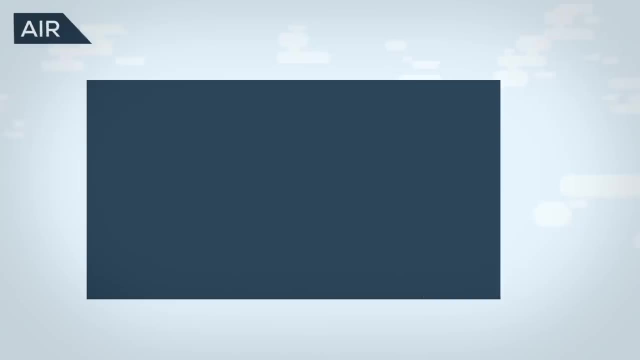 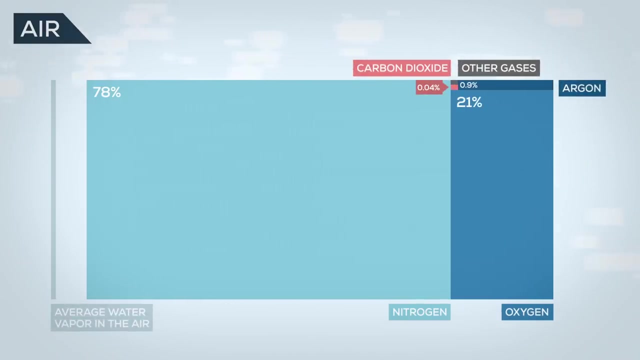 But don't let us fool you into thinking we have it all figured out. Speaking of breathtaking information, what about the airy stuff that surrounds us? By volume, dry air consists mostly of nitrogen, oxygen, argon, carbon, a variable amount of water vapor and small amounts of other gases. 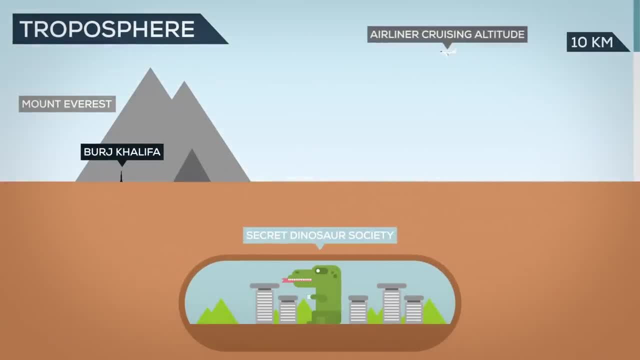 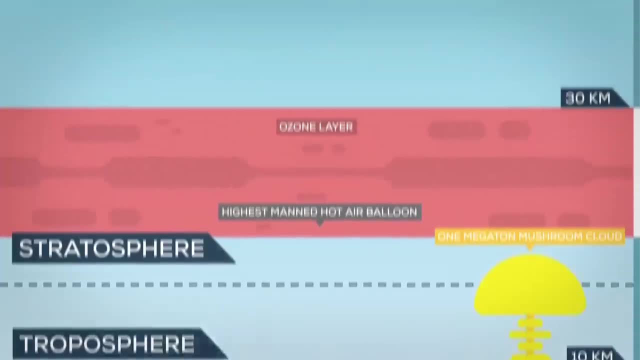 Humans are very dependent on the lowest layer of the atmosphere, the troposphere, where the weather is. It's 12 kilometers thick on average. Above that is the stratosphere, which is where the ozone layer protects us from the sun's most aggressive type of light. 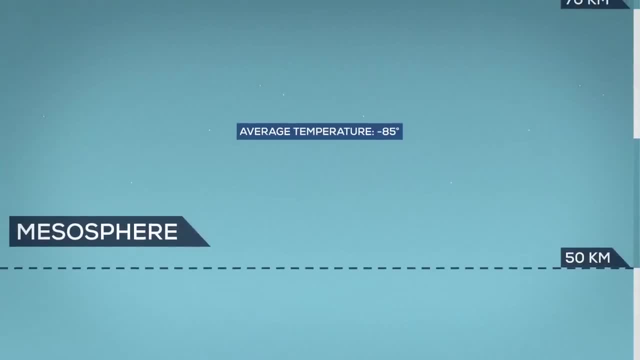 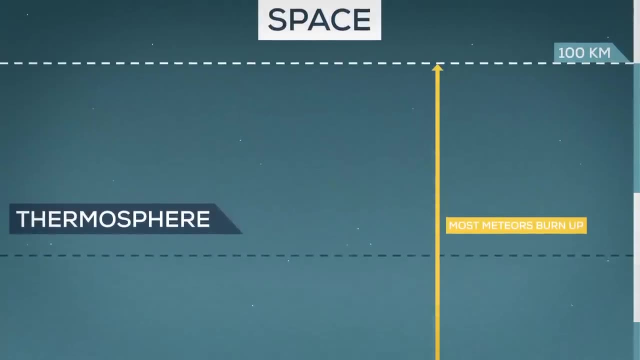 Above, that is the mesosphere, the coldest place on Earth, with an average temperature around minus 85 degrees Celsius. At about 80 kilometers up, the thermosphere starts. The transition to space is a fluent one, without clear borders, But humans are not. 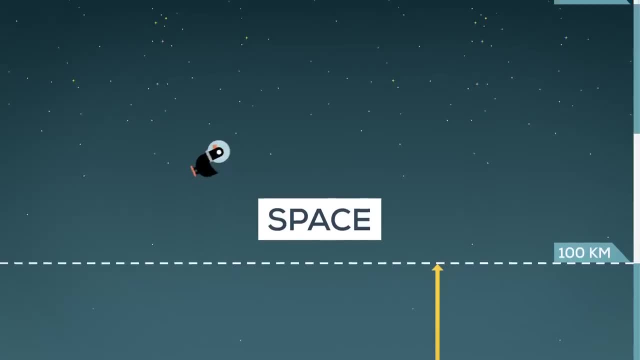 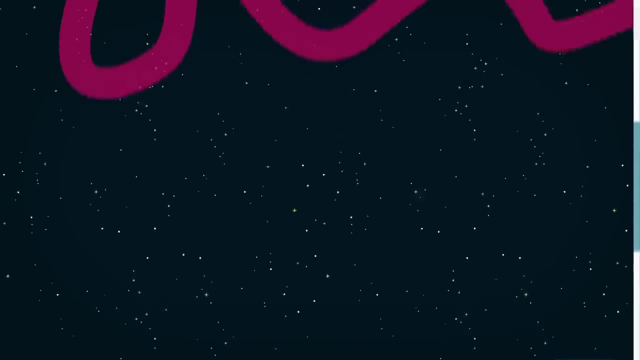 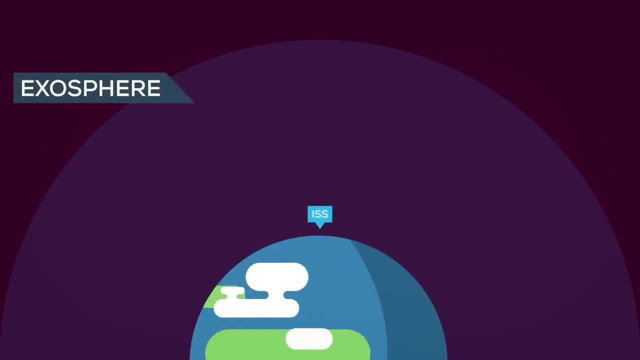 Humans decided that space starts here. At about 100 kilometers, Earth stops and space begins, though the atmosphere extends a bit further. In this region we find the ionosphere, the aurora borealis and the ISS, And the outermost layer is the exosphere stretching up to 10,000 kilometers.